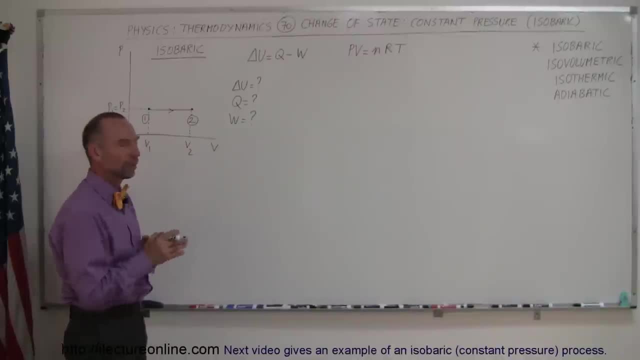 videos, but right now we're only going to talk about the isobaric one, That means the constant pressure one, And so in each case we're going to try to figure out what the change of the internal energy is, what the heat added to the gas is and what the work done by the gas is. So the change in the temperature is called the isobaric change of phase. Matter of fact, constant pressure is called isobaric change of phase. So if you're going to say in this case the constant pressure is called constant temperature, We know that the constant temperature is usually pretty straightforward. 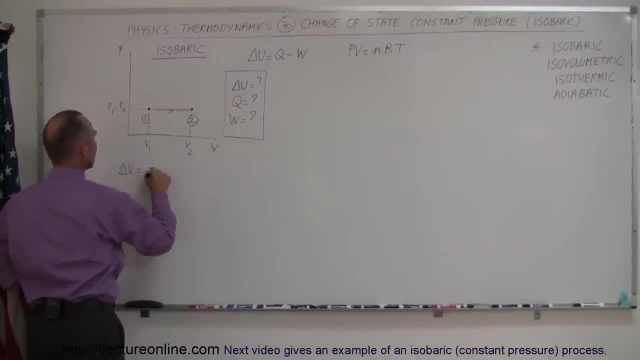 we know that delta U is always going to equal N C sub V times delta T. Now, of course, if you don't know what the delta T is, then you're not going to be able to figure that out directly. but at least that's a start. that's how we typically do it. Q can be figured out by saying: 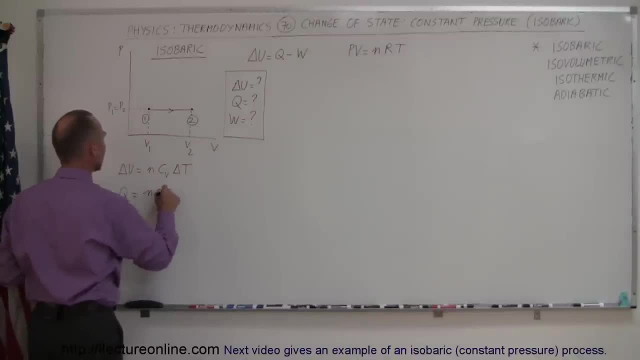 well, in this case, since the pressure is constant, this is going to be N C sub P, delta T. But again, if you don't know what the delta T is, you may have trouble figuring it out. So hopefully that's figuring out what the Q is in this case. And finally, we know that work since its constant. 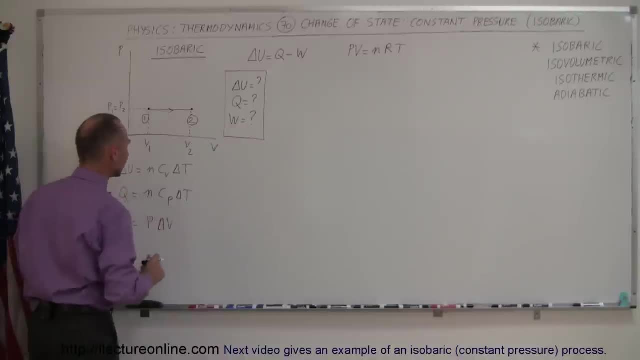 pressure can be written as P times delta V, and of course, if you know the beginning and ending volume and you know the pressure, then that would be straightforward. Then you combine that in conjunction to the first law of thermodynamics, which says that the change in internal energy is 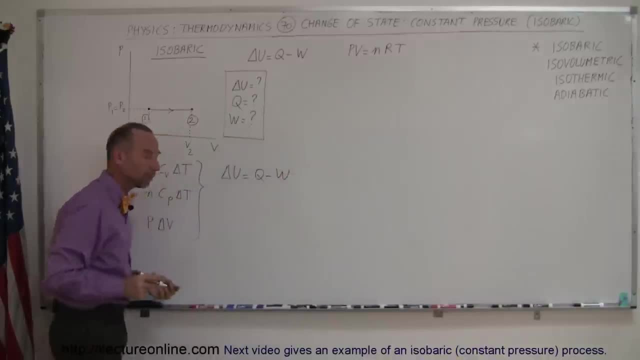 equal to Q minus W. So sometimes it will actually tell you how much heat is added or taken away from the gas, and if you then calculate what the work done is, you can then go back and find the internal energy. So there's usually a combination of ways in which you can figure that out Now. 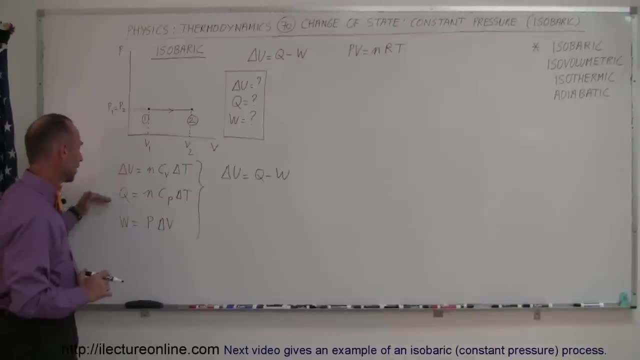 let's see here. So we have the internal energy change, we have the heat added or taken away and we have the work done by the gas. Now what you can also look at is where you started and where you ended up. If you go to the right or you go upward, then the temperature will always. 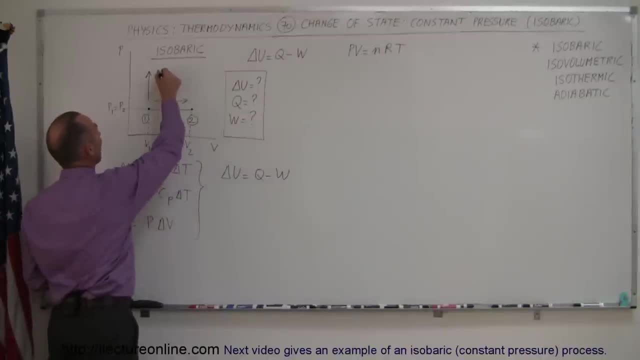 increase. So if you go to the left or you go upward, then the temperature will always increase. So this indicates a positive delta T. So in this case, when we went from one to two and the volume increased, that means the temperature will also increase If you go. 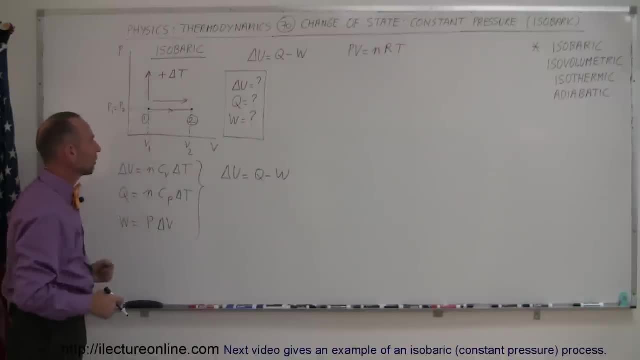 from here to a higher pressure state, then you also know that the temperature will increase. If you go from right to left, you know the temperature will decrease. If you go up to down, you know the temperature will decrease. In addition, we could also find out the work done by figuring out the 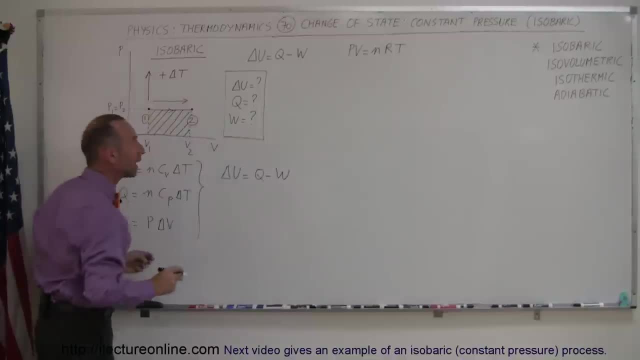 area of the curve underneath the line that represents the change in state. So we can also say that the work done, work done is equal to the area. work done is equal to the area under the curve. All right, so now let's say we have an example, and I think I have some, a nice little. 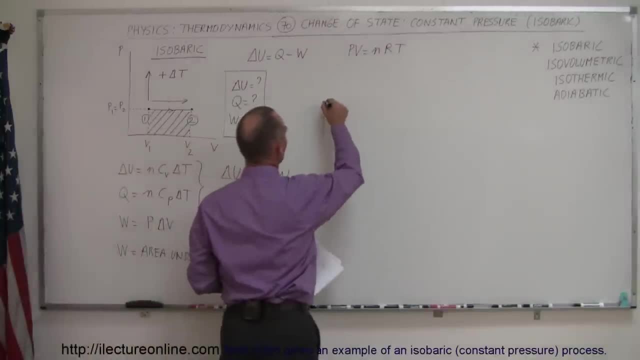 example for us here. Let's say that we start out with a gas like so, and let's say that the initial pressure- pressure initially- is equal to 1.5 atmospheres, And let's say that the volume- volume initial- is equal to 15 liters, L for liters- And let's say that 800 energy of joules leaves the gas. 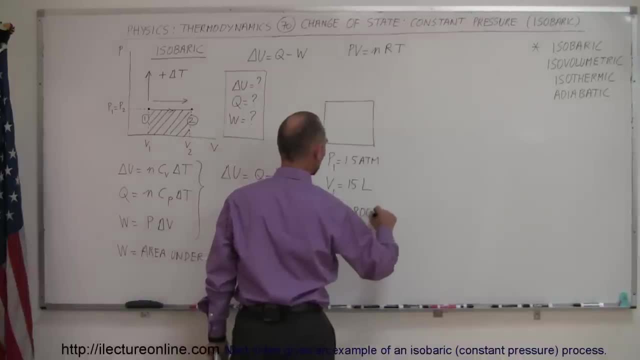 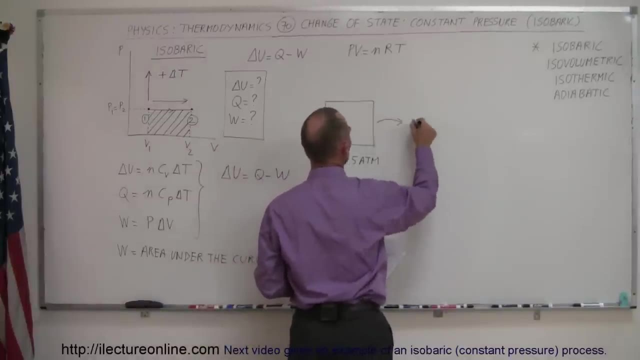 So Q is equal to minus 800 joules. Based upon that, oh, we also need to have a final state. So that's the initial state. Let's say that it changes to minus 800 joules. So Q is equal to minus 800 joules. 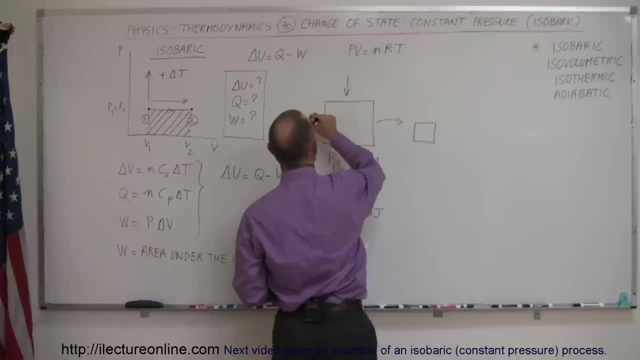 It changes to a final state, which means that the gas is being acted upon by its surroundings. It's being compressed, The pressure final. the second state of the pressure is equal to. I don't have that. Let's see here. Volume two is equal to two liters, So it's being compressed down to two. 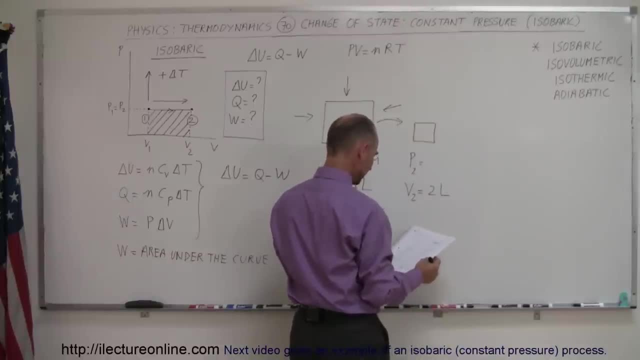 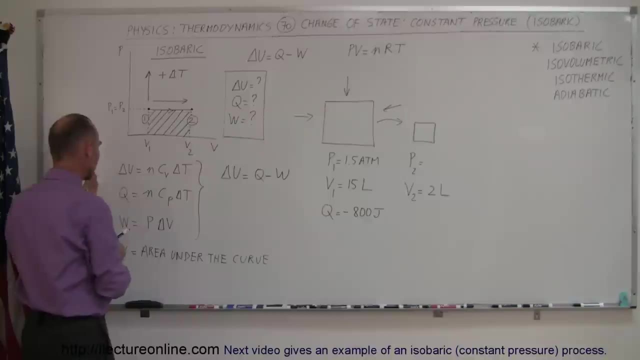 liters, And that's it. They don't give us any other information. Can we figure out these three quantities right here, the change in terms of the pressure and the change in terms of the internal energy, Q and W. based upon that? So well, let's see here. I think I do know what final 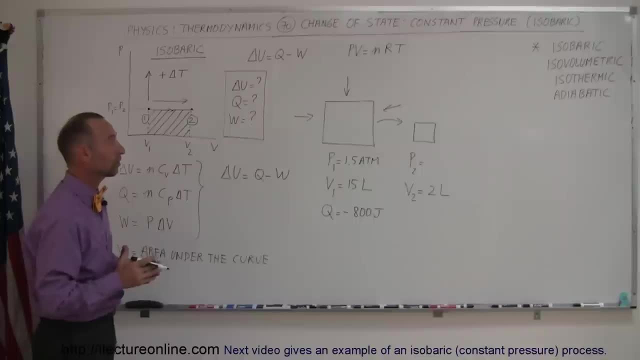 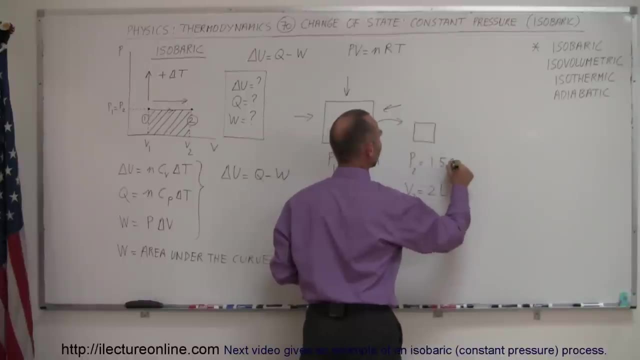 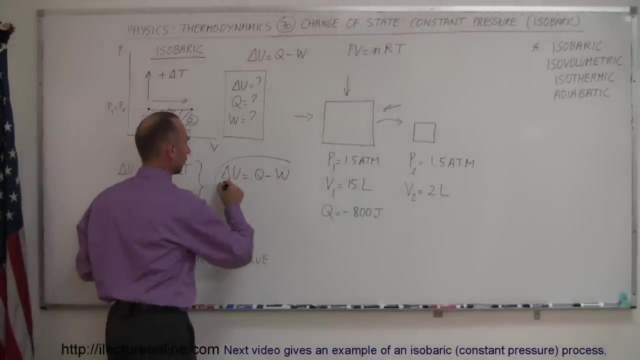 pressure is because we're in the case here where we have an isobaric process. Isobaric process means that the pressure doesn't change, So therefore, we also know that this has to be 1.5 atmospheres. All right, So that's case one. Now, secondly, we're going to use our second law of thermodynamics. 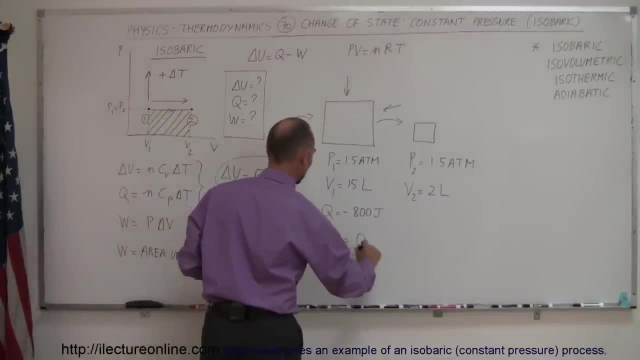 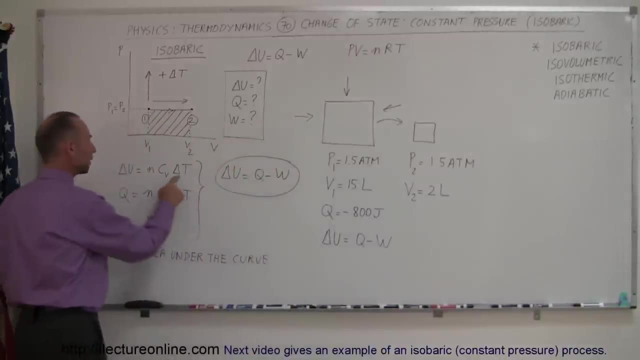 We're going to say that delta U is equal to Q minus W. Now notice that I cannot directly figure out what delta U is because I don't know my change in temperature. I didn't get the initial or final temperatures. I do know what Q. 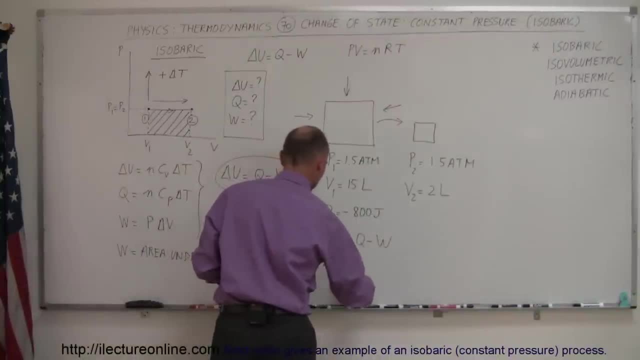 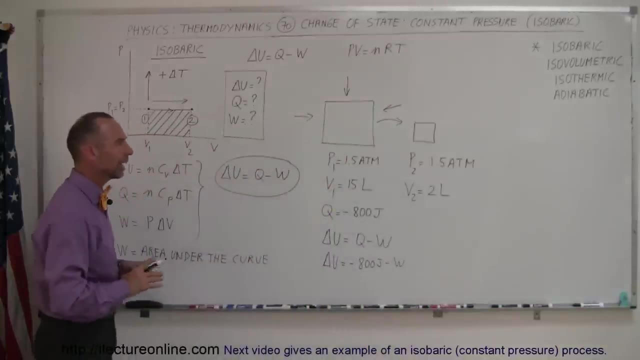 is, It's minus 800 joules. So delta U is equal to minus 800 joules, minus W. Now, secondly, can I find out what W is? And the answer is yes, because I know my pressure, which doesn't change, and I. 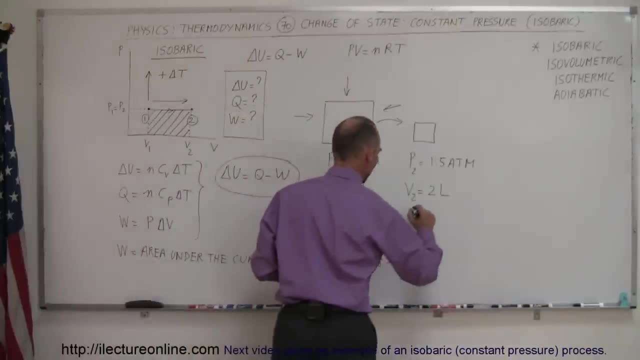 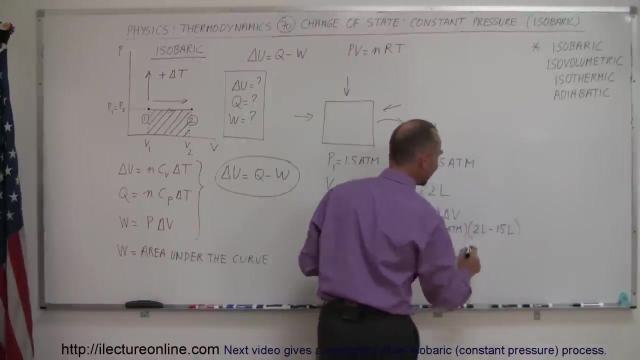 know the change in volume, So I can say that the work done is equal to pressure times delta V, And so it's equal to 1.5 atmospheres times the delta V. The final volume is 2 liters. The initial volume is 15 liters. So we can see. 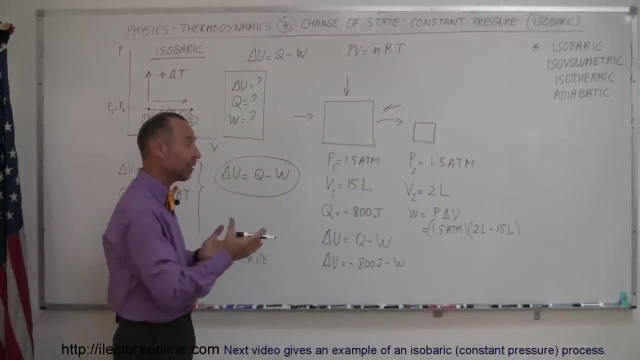 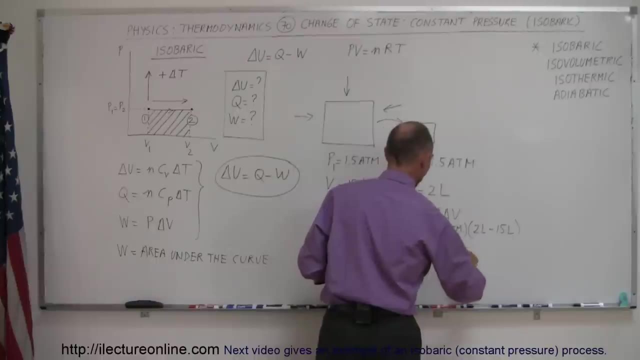 that the change in the volume is a negative 13 liters. Negative volume change means negative work done. So this is equal to 1.5 times 101,300 pascals, Because we have to convert two standard units And of course there's 1,000 liters in the cubic. 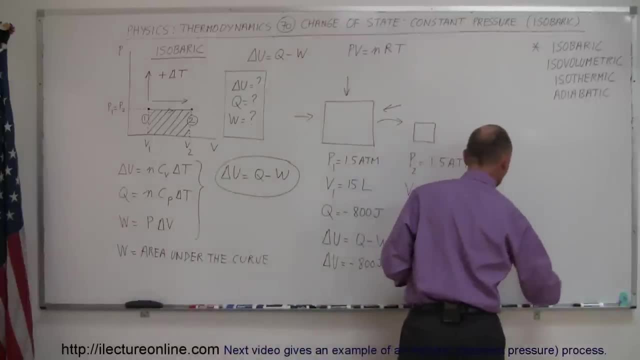 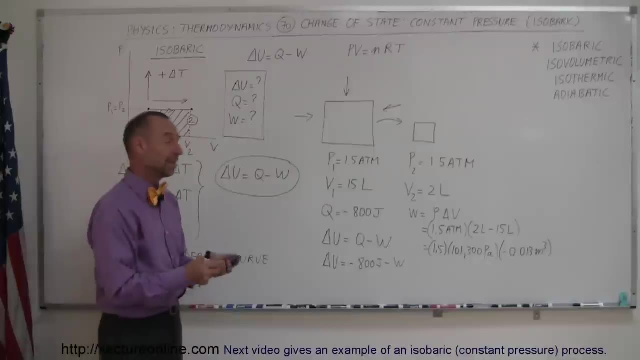 meter. So minus 13 liters is minus 0.013 cubic meters, And so that gives me the work done by the gas, And since it's negative, that means it's going to be worked on on the gas. So we have 1.5. 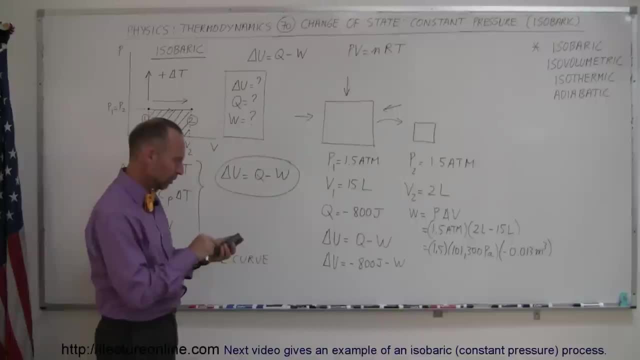 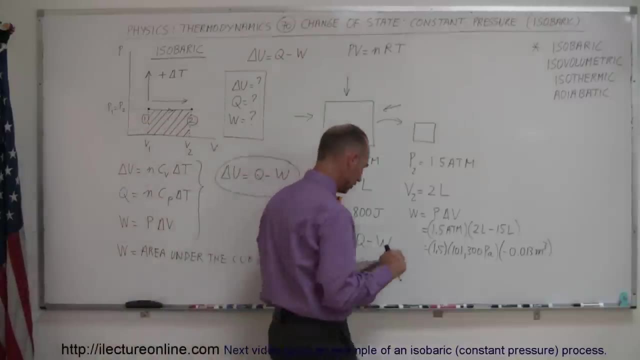 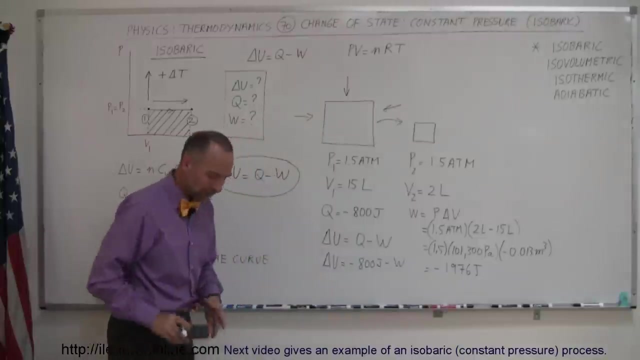 times 101,300.. Oop, one too many zeros- 101,300.. And then times 0.013 equals, and it looks like it's going to be a minus 1,976 joules. All right, So now what I have is: I have the heat added to the. 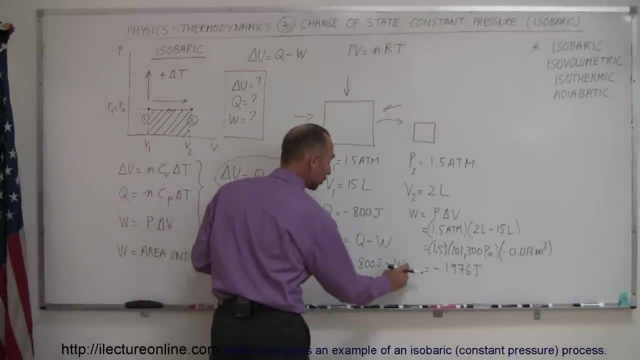 gas which is negative, which means it's actually removed from the gas. I have the work done by the gas which is negative, which means actually work is done on the gas. And since I now know these two quantities, I can also figure out the change in internal energy. So delta U is equal to minus. 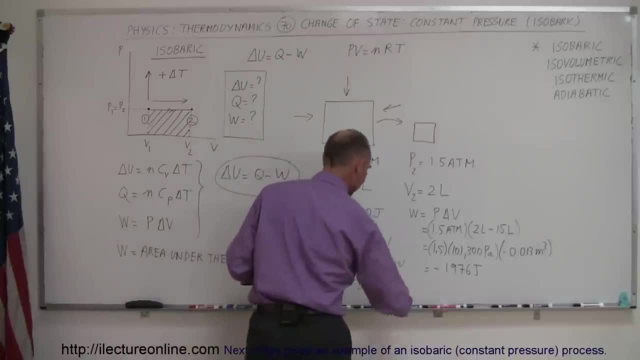 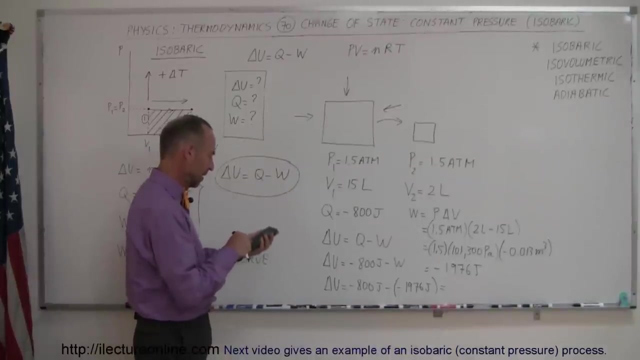 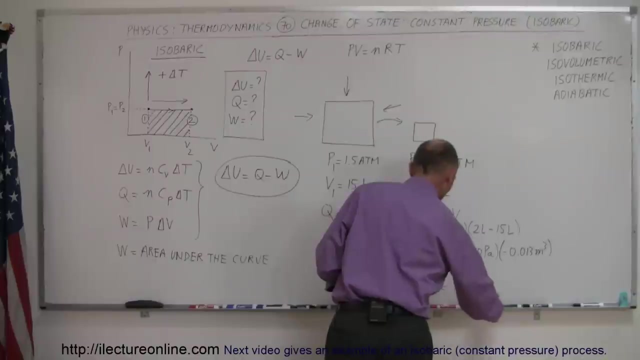 800 joules, And then it's a minus. Huh, that's interesting. Now, minus times a minus. So we have to be very careful with the signs. Minus times a minus 1,976 joules. So finally we have 1,976 minus 800 equals 1,176.. 1,176.. And it's positive, which means that